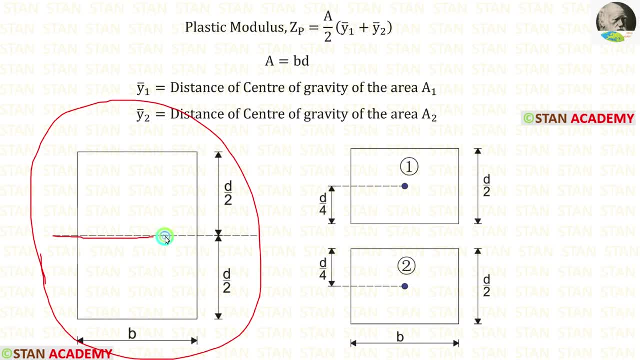 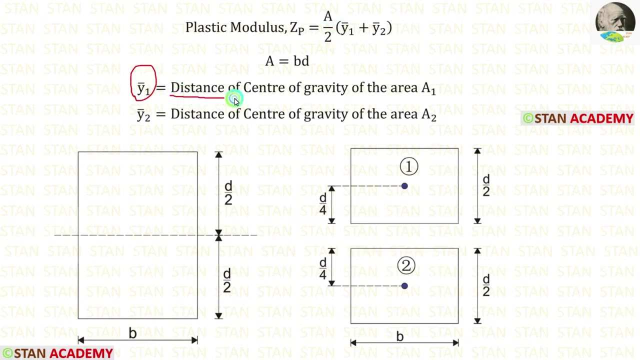 is symmetrical, so the equal area axis lies in the center. So we have to split the rectangle into two parts, above the equal area axis and below the equal area axis, y1 bar is equal to the distance of center of gravity of the area a1.. y2 bar is equal to the distance of center of 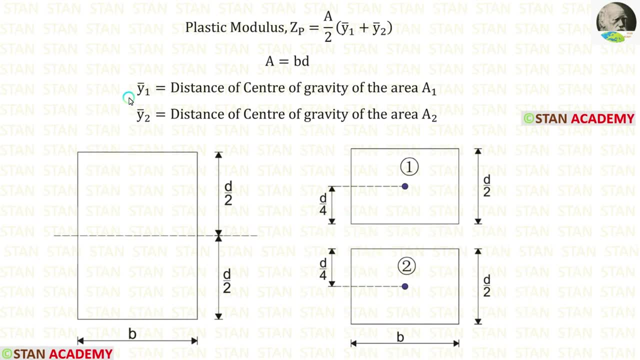 gravity of the area a2. Here we have to be very careful. We have to calculate y1 bar and y2 bar from the equal area axis. You can see that I am calculating y1 bar from the equal area axis. For the second, 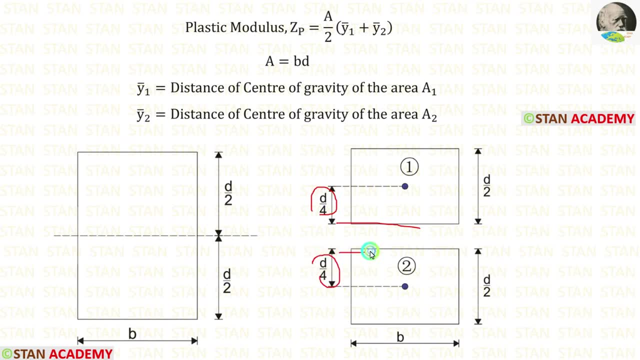 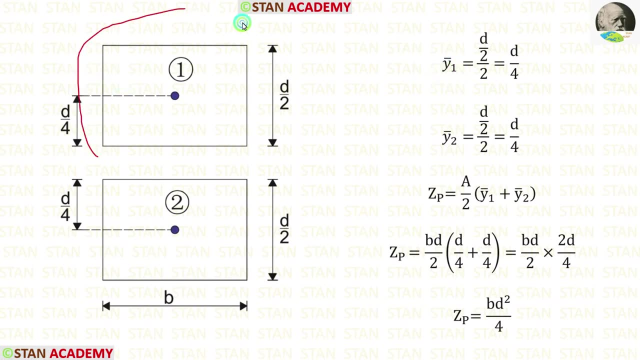 part. also, I am calculating y2 bar from the equal area axis. Now let us calculate y1 bar. This rectangle is symmetrical, so the centroid lies in the center. So we have to calculate the center of d by 2.. d by 2 by 2. 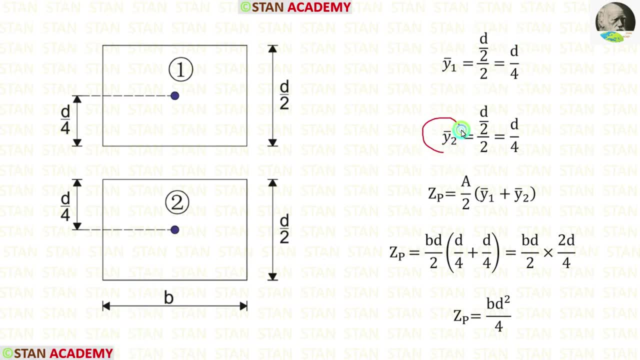 we will get d by 4.. In the same way, we have to calculate y2 bar for the second rectangle. Here also, we are getting d by 4.. Now let us calculate the plastic modulus. We can apply the values inside the formula Area. we have already calculated bd, Now we can the apply. 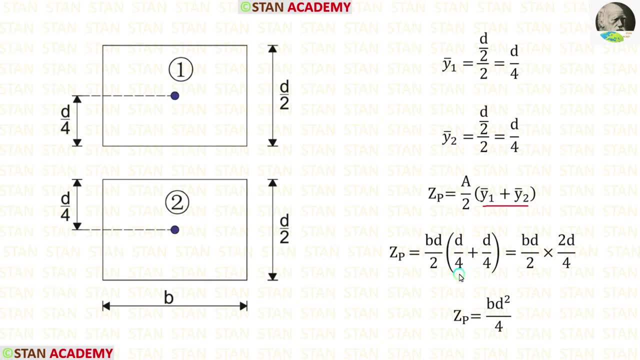 values of y1 bar and y2 bar. d by 4 plus d by 4, we will get two. For d by 4 plus d by 4, we will get d by 4 into central d and D is equal to d by 4.. We can cut this 2 and 2.. Finally, we are getting: zp is equal to bd square by 4.. 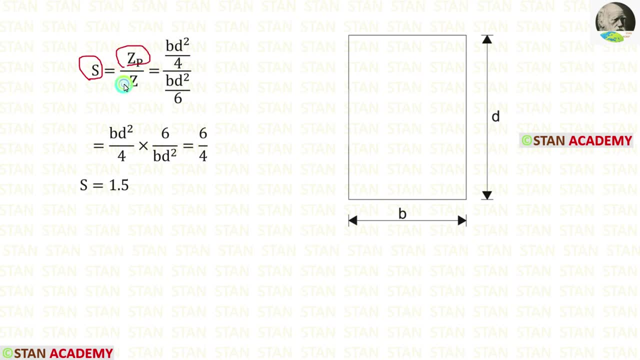 In the shape factor formula. we have calculated zp and z. We can apply the values, We can cut bd square and bd square. Finally, we are getting 6 by 4.. 6 by 4 is equal to 1.5.. 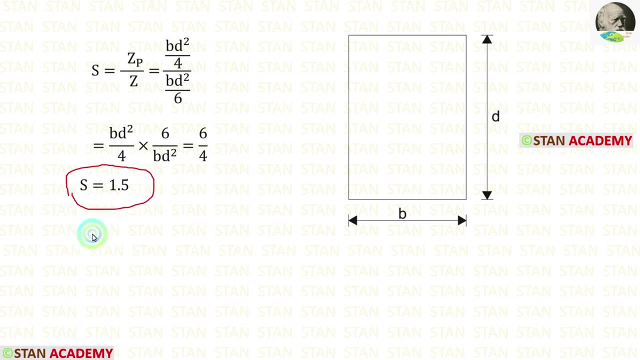 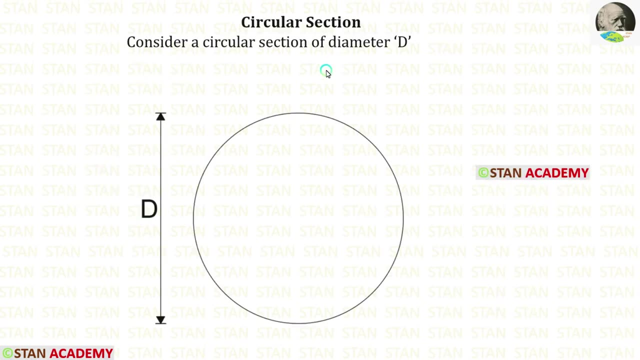 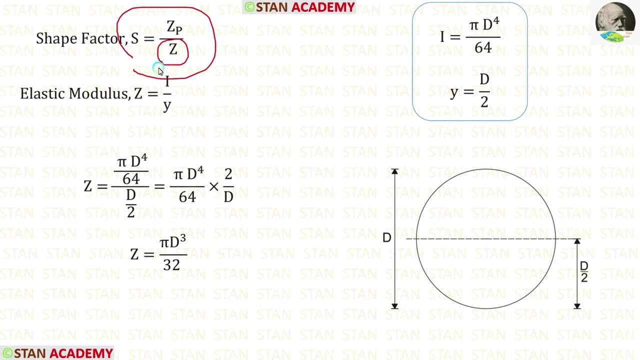 Finally, we have calculated the shape factor for a rectangular section, which is equal to 1.5.. Now let us calculate the shape factor for a circular section. Consider a circular section of diameter d In the shape factor formula. first let us calculate the elastic modulus z. The formula for elastic modulus is equal to i by y. 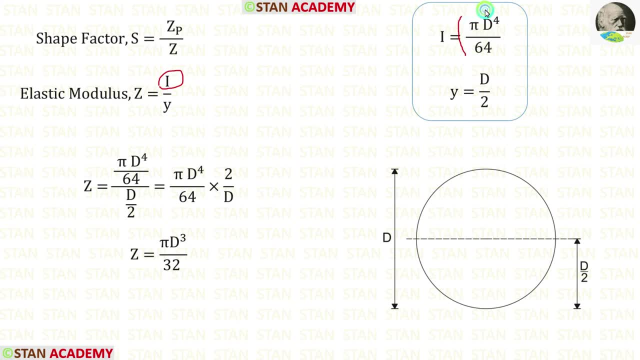 The movement of inertia for a circular section is equal to pi d power 4 by 64.. The circle is symmetrical, So the neutral axis lies in the center. From the center the distance is d by 2 to the 5-bar, So y is equal to d by 2.. In the formula we can apply the values: 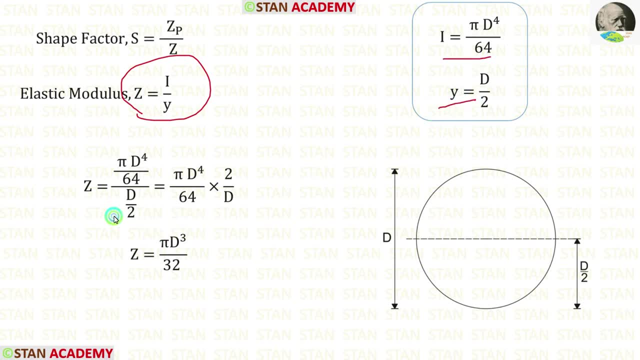 of movement, of inertia and y. can take d by 2, inversely, and multiply. We can cut 2 and 64. Here it will be 32.. Also, we can cut d and d power 4. Here it will be 3.. Finally, we are getting: z is equal to pi, d power 3 by 32.. 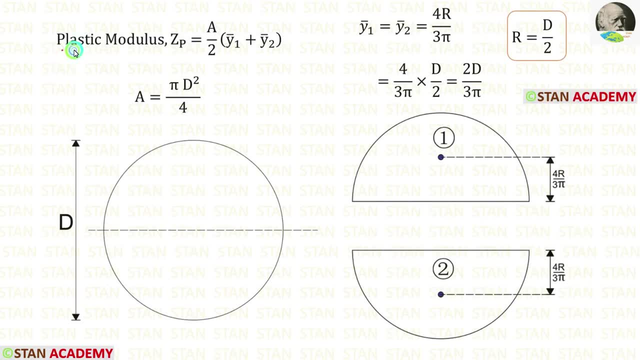 Now let us calculate the plastic modulus zp. The formula is a by 2 into y1 bar plus y2 bar. For a circle, the area formula is pi d square by 4.. For calculating y1 bar and y2 bar we have to: 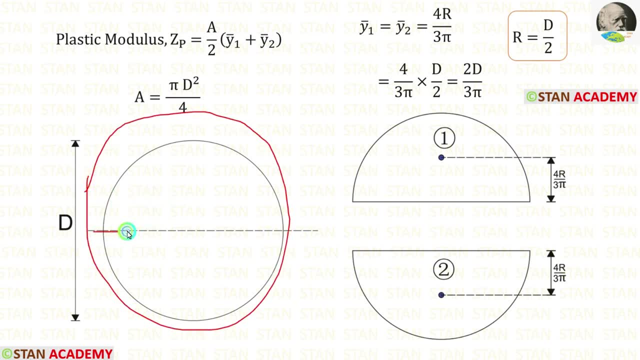 split the circle into two parts about the equal area axis. This circle is equal to pi d square by 4.. Now let us calculate the plastic modulus zp. The formula is a by 2 into 4.. So the equal area axis lies in the center. Let us split the circle into two parts about the 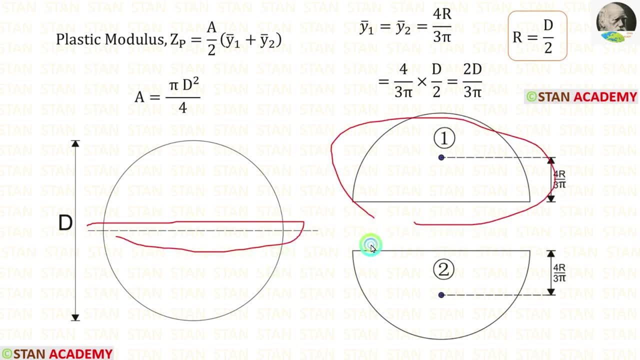 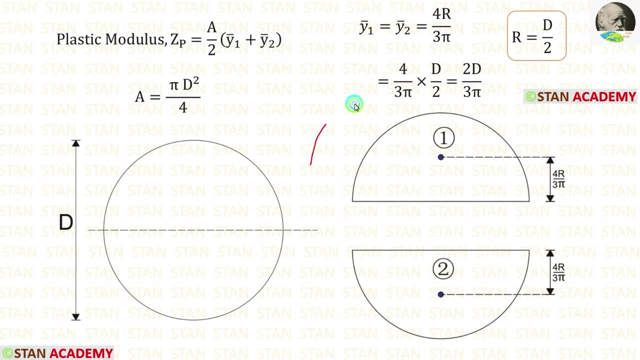 equal area axis, One above the axis and one below the axis. Now let us find the location of the centroid. For the first part, the centroid lies at a distance of 4r by 3 pi from the bottom. For the second part, the centroid lies at a distance of 4r by 3 pi from the top, So y1 bar is equal to y2 bar.